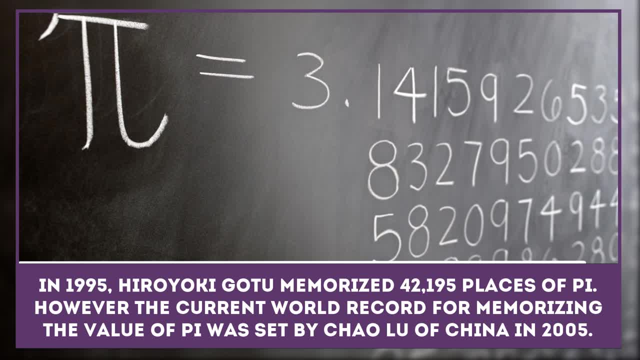 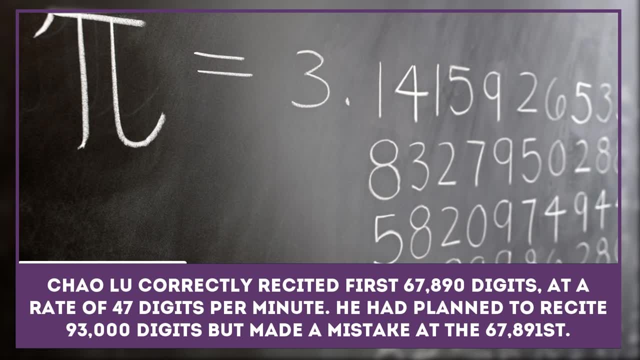 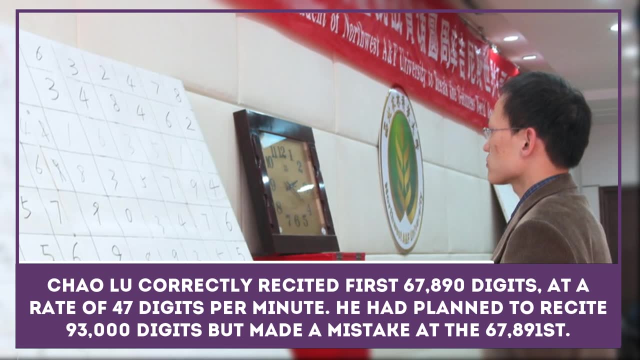 Japanese is better suited than other languages for memorizing sequences of numbers. However, the current world record for memorizing the value of pi was set by Cao Lu of China in 2005.. He correctly recited from memory its first 67,890 digits. 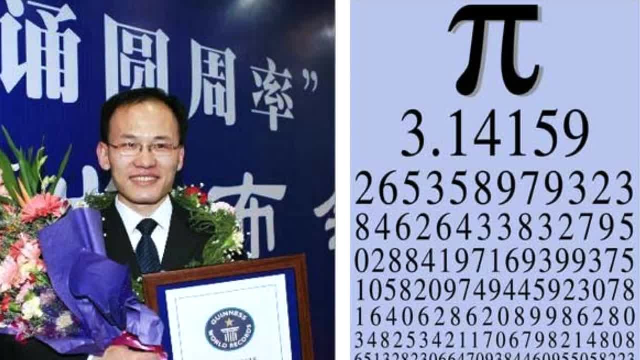 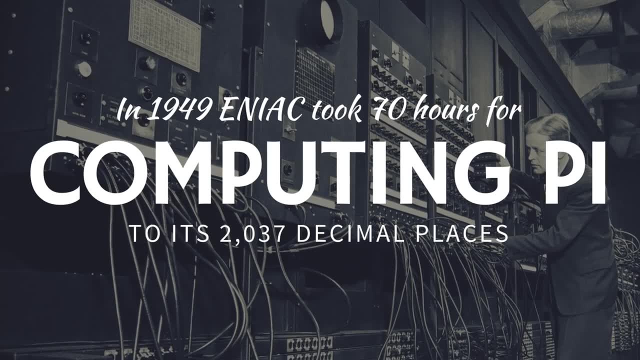 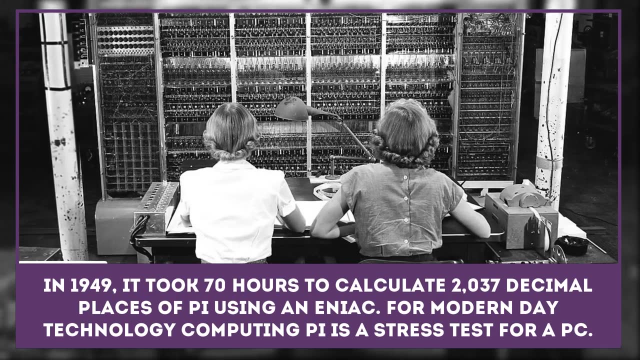 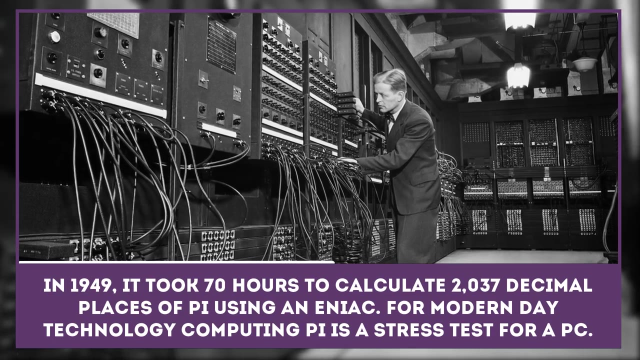 at a rate of 47 digits per minute. In 1949, it took 70 hours to calculate 2037 decimal places of pi using an electronic numeric integrator and computer. For modern day technology, computing pi is a stress test for a computer. 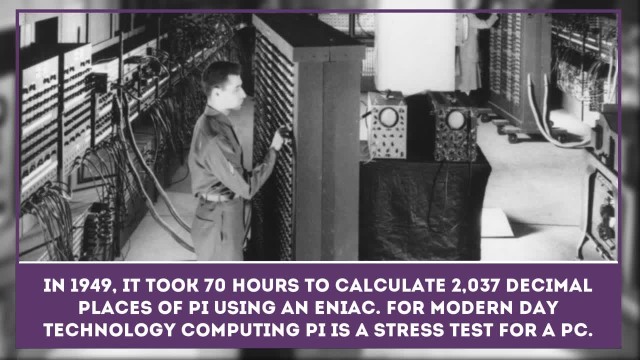 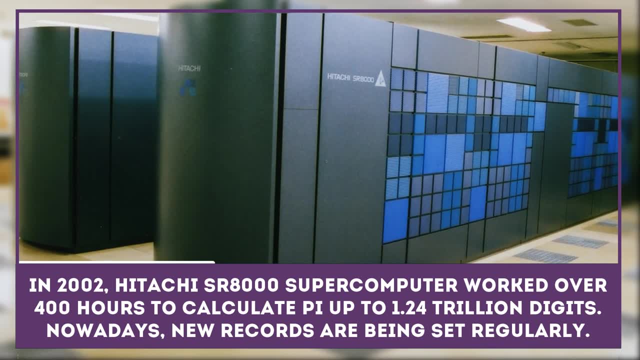 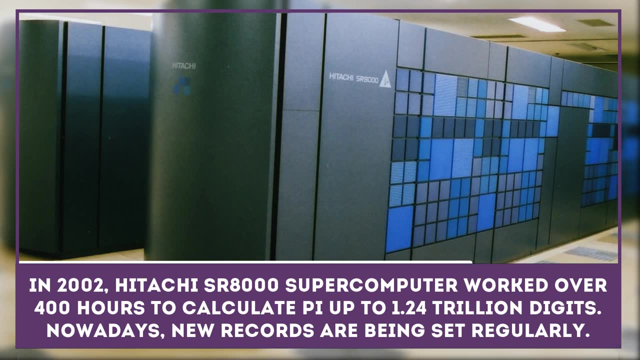 A kind of digital cardiogram. In 2002, Hitachi SR8000 supercomputer worked over 400 hours to calculate pi up to 1.24 trillion digits. Nowadays, new records for calculating pi are being set regularly. As of 2010,, the record is 5 trillion digits. 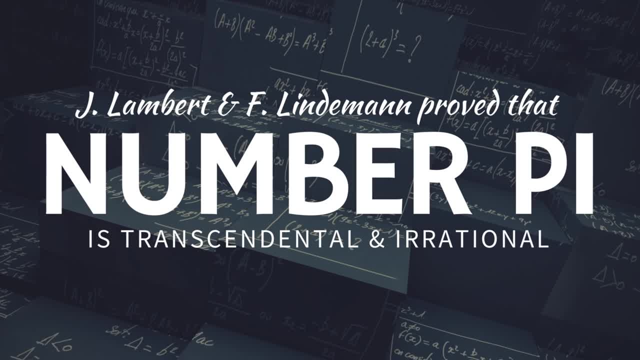 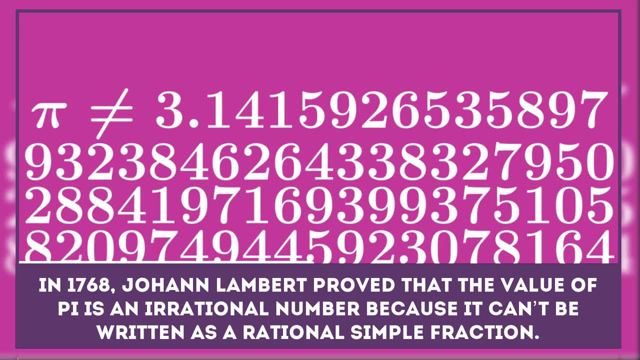 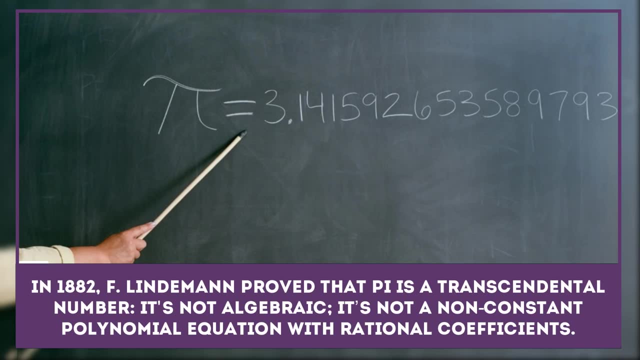 In 1768, Johann Lambert proved that the value of pi is an irrational number because it can't be written as a rational simple fraction. In 1882, Ferdinand Lindemann proved that pi is a transcendental number because it is not algebraic. 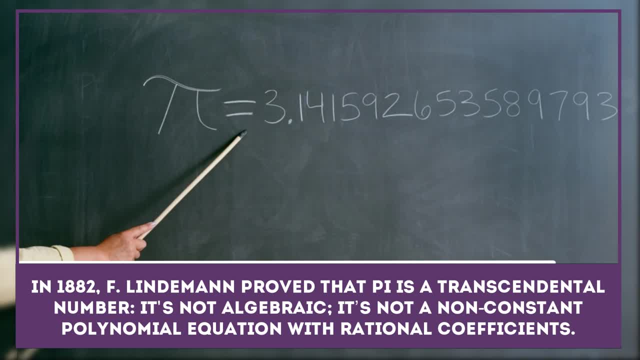 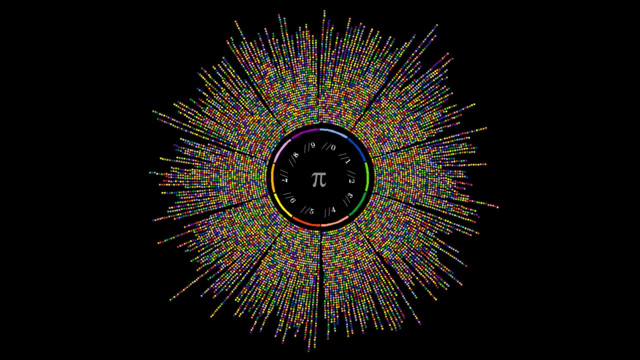 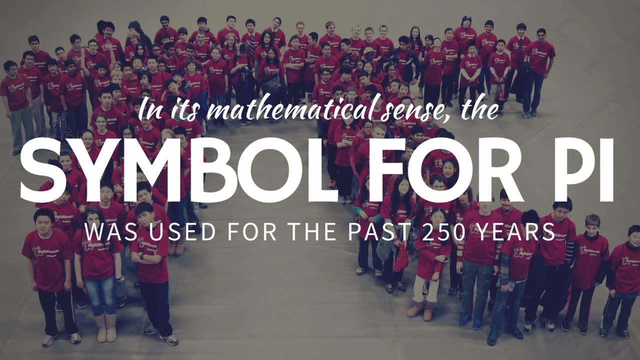 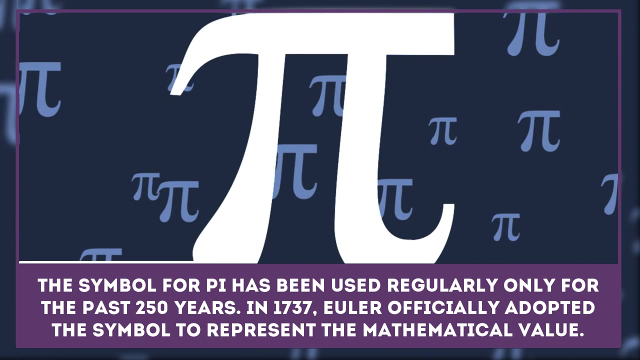 It's not a non-constant polynomial equation with rational coefficients. Pi is a number that can't be written as a real number. because it can't be written as a real number, The symbol for pi has been used regularly in its mathematical sense only for the past 250 years. 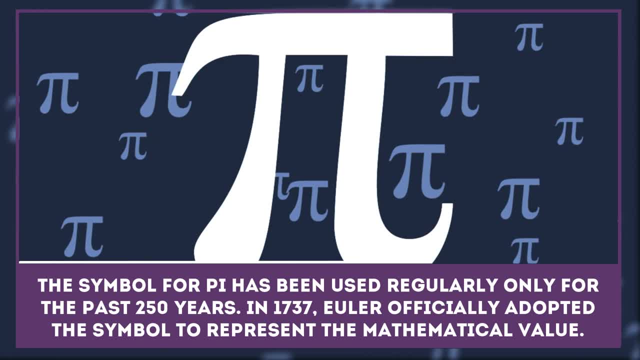 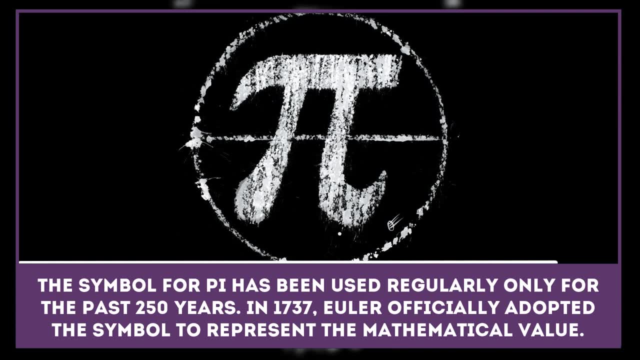 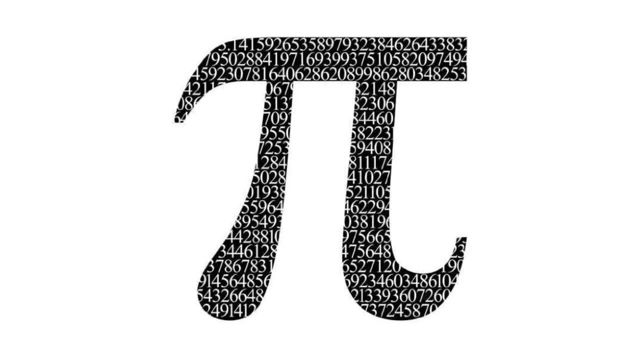 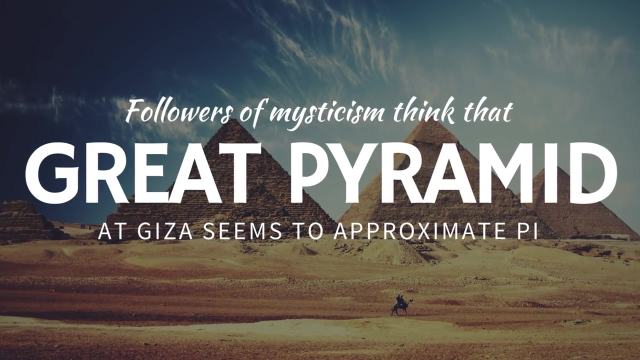 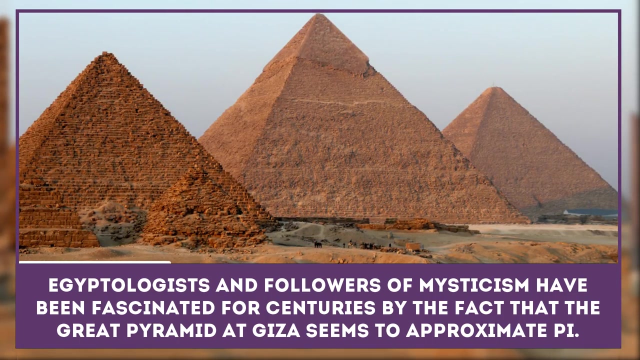 In 1706, an English mathematician introduced the Greek alphabet pi to represent the said value. However, in 1737, Euler officially adopted this symbol to represent the value. Egyptologists and followers of mysticism have been fascinated for centuries by the fact that the Great Pyramid at Giza seems to approximate pi. 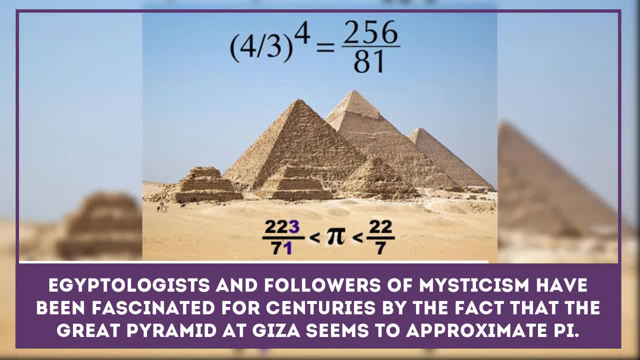 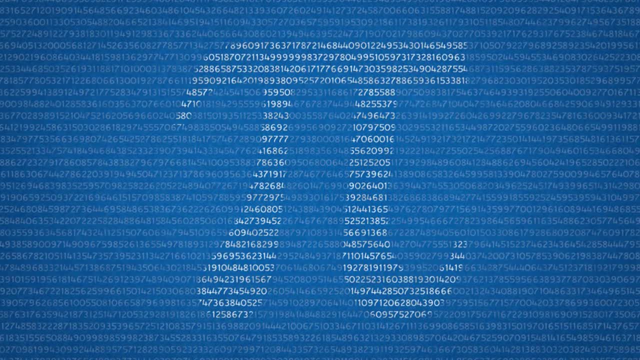 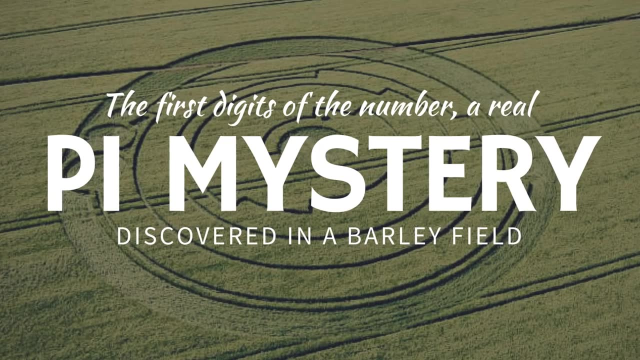 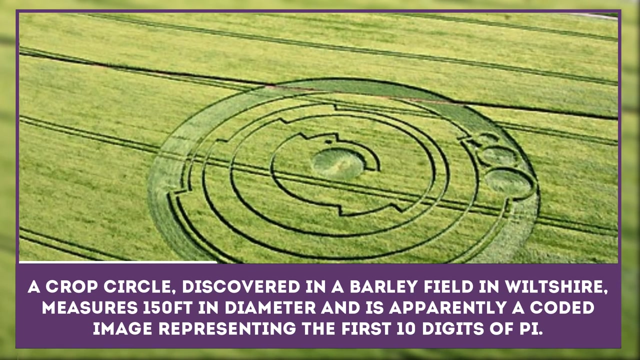 The vertical height of the pyramid has the same relationship to the perimeter of its base as the radius of a circle has to its circumference. The most complex, mind-boggling crop circle ever to be seen in Britain has been discovered in a barley field in Wiltshire. 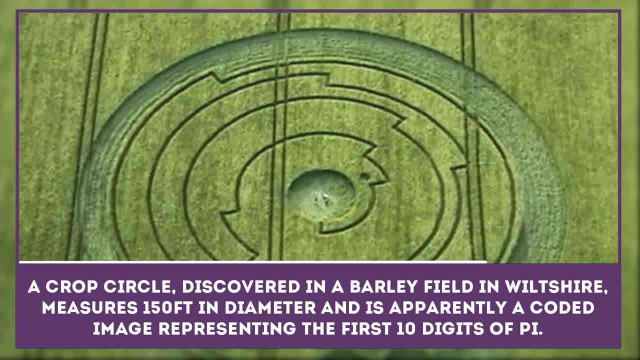 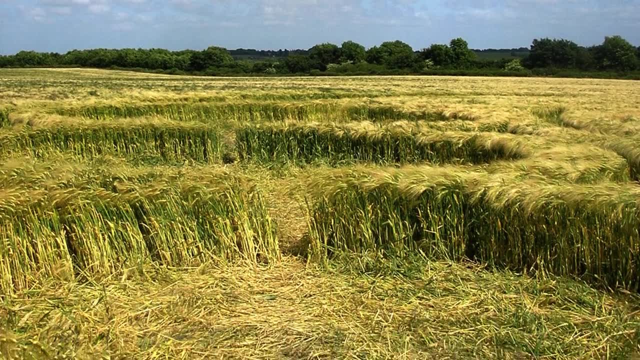 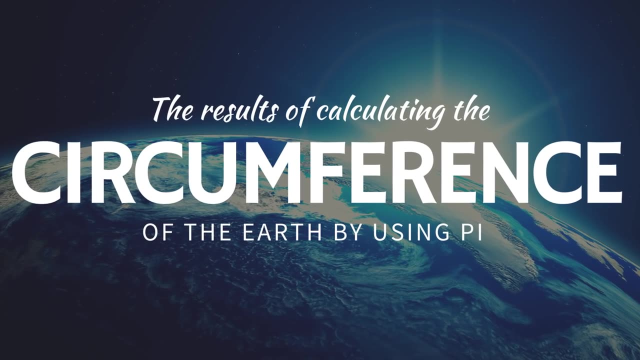 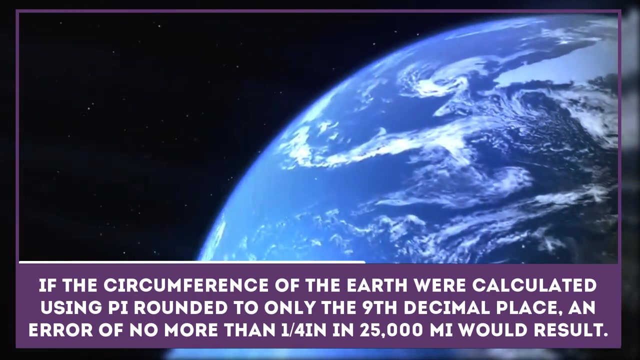 The formation measuring 150 feet in diameter is apparently a coded image representing the first ten digits of pi. If the circumference of the Earth were calculated using pi rounded to only the ninth decimal place, an error of no more than one quarter of an inch in 25,000 miles would result.